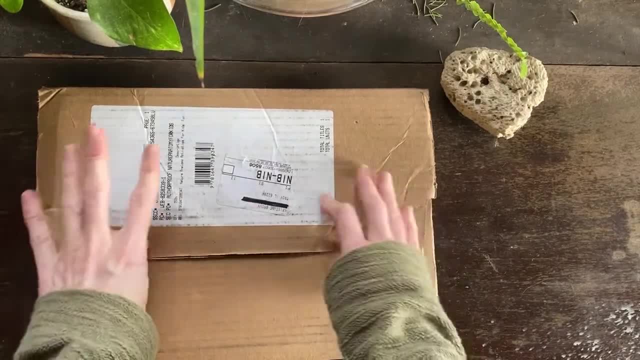 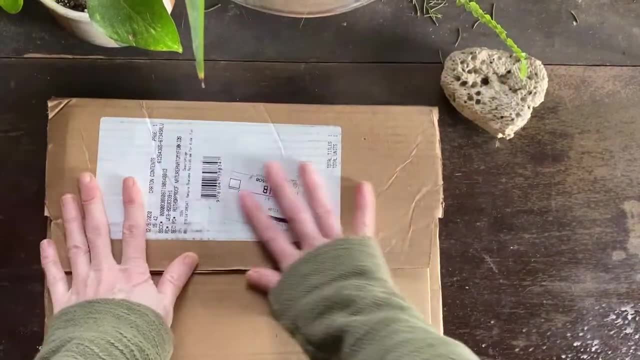 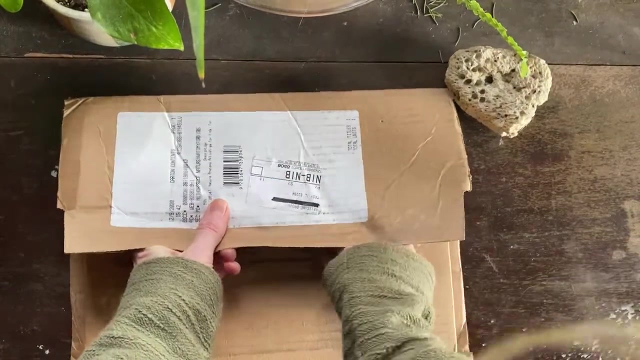 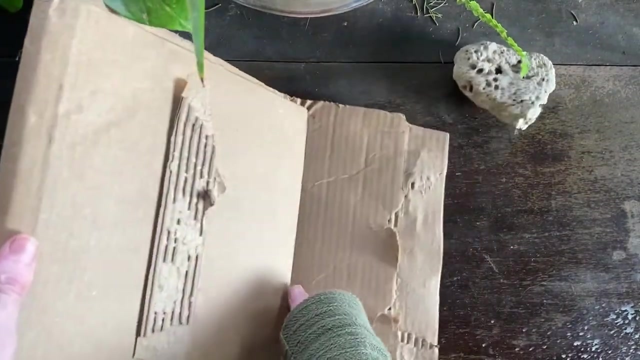 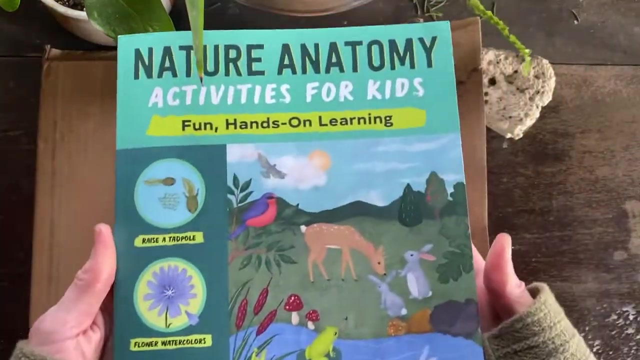 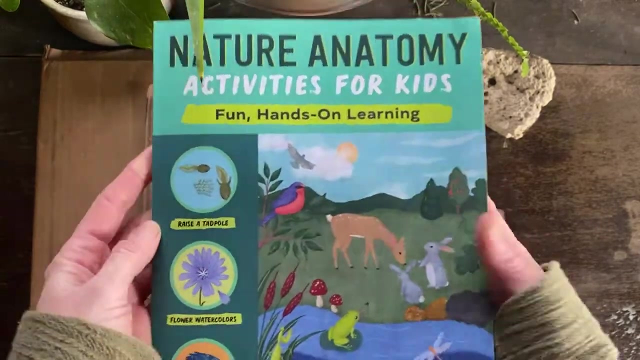 Today was a happy mail day. I received a copy of my author proof of my newest book, so I'm going to open it up and show you what it looks like. I'm just so happy with it. So it's Nature, Anatomy Activities for Kids, Fun, Hands-on Learning, And I just love the colors and the illustrations. The artist did a wonderful job with this book. 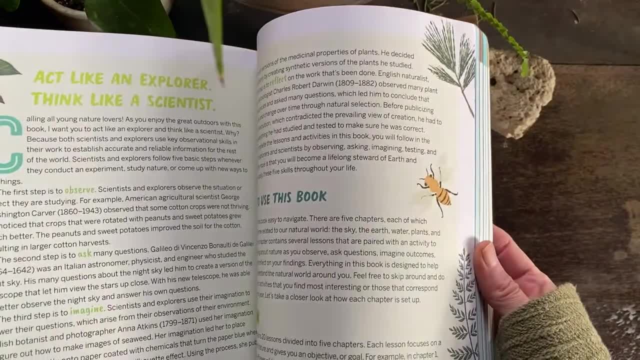 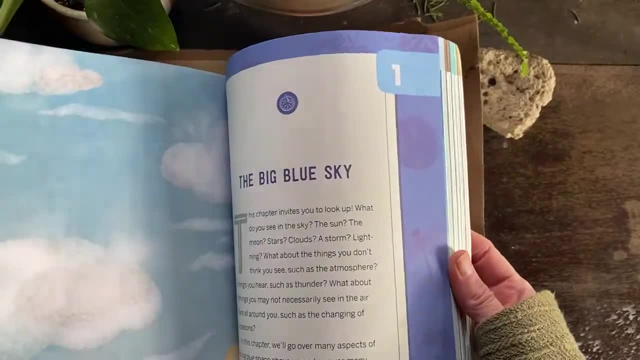 And it's going to teach your kids to act like an explorer and think like a scientist, And so this book begins with showing some how-tos- how to get the most use out of this book- And then I'm going to open it up and show you what it looks like. I'm just so happy with it. So it's Nature, Anatomy Activities for Kids, Fun, Hands-on Learning, And I just love the colors and the illustrations. The artist did a wonderful job with this book. 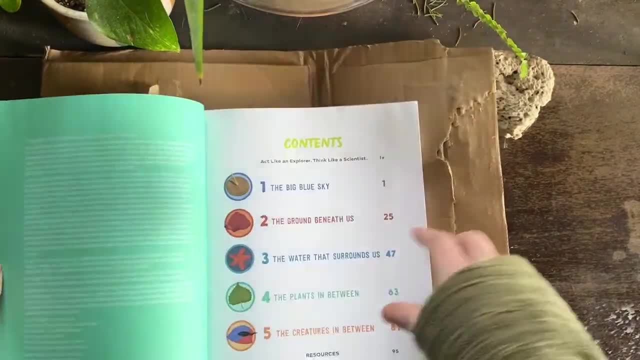 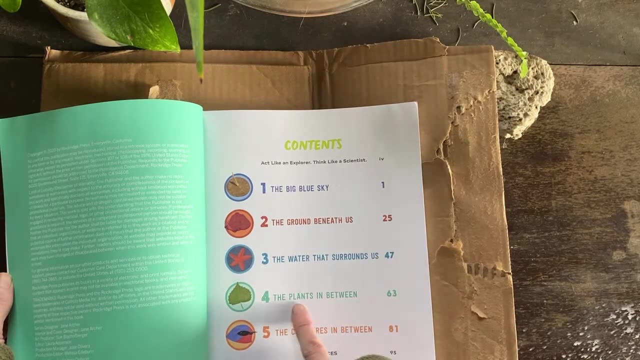 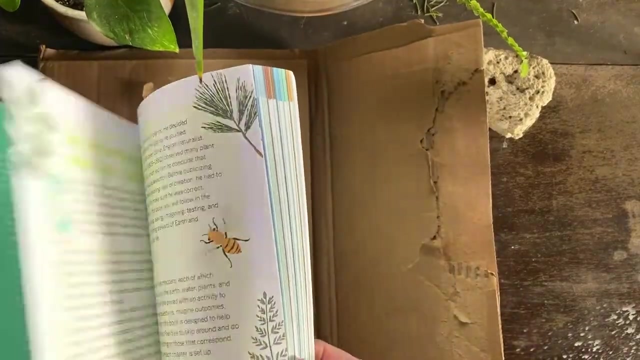 And then there are five sections. So we have the big blue sky, the ground, Meninas, the waters that surrounds us, the plants in between and the creatures in between. So it starts out with all kinds of adventure activities for things that happen in the sky. 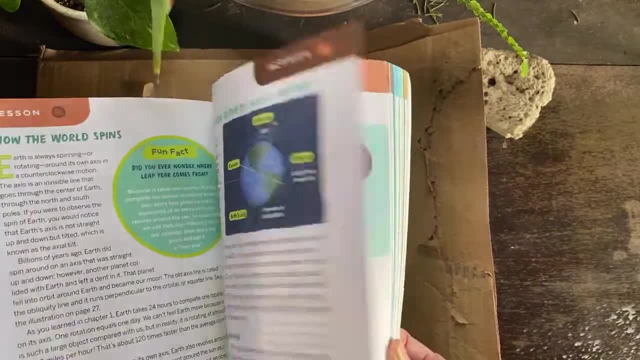 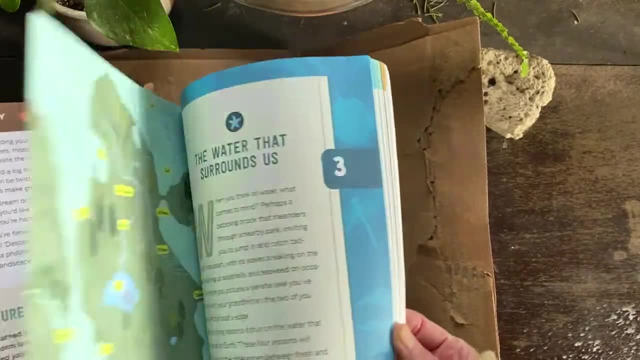 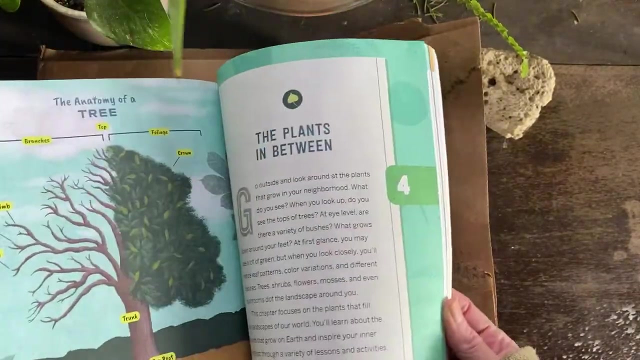 And then we move down to the earth and we look at all the things in the earth, what it's made of, How land is formed, And then it takes a look at all the types of waters around us And moves on to my favorite topic: plants. 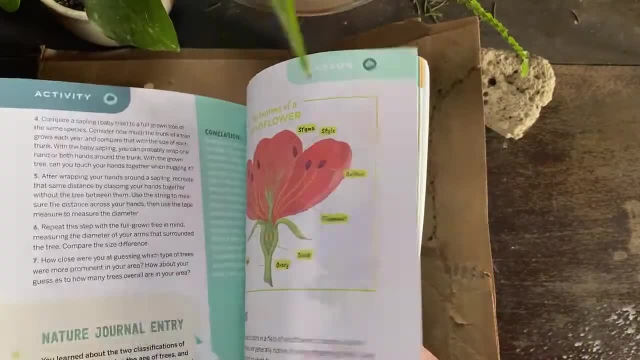 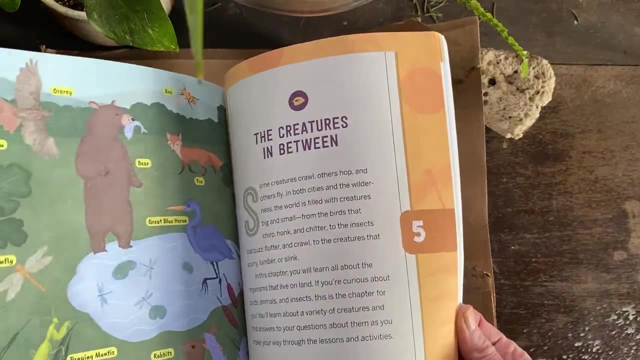 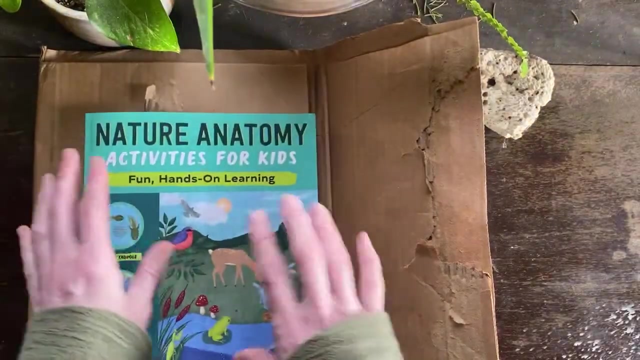 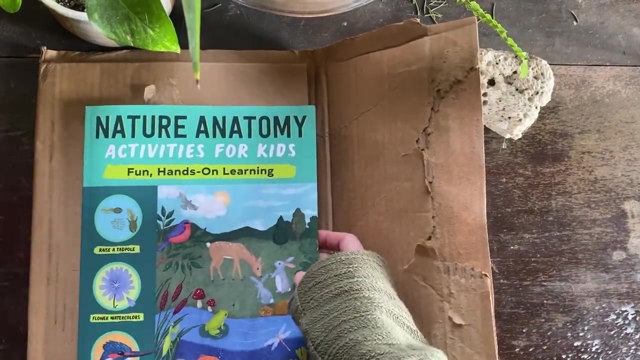 And shows some fun plant activities, And then finally the creatures in between, And then finally the creatures in between. It's just a lovely little book. I just love how it's put together. It contains 20 different activities, And each activity is accompanied by a journal entry. 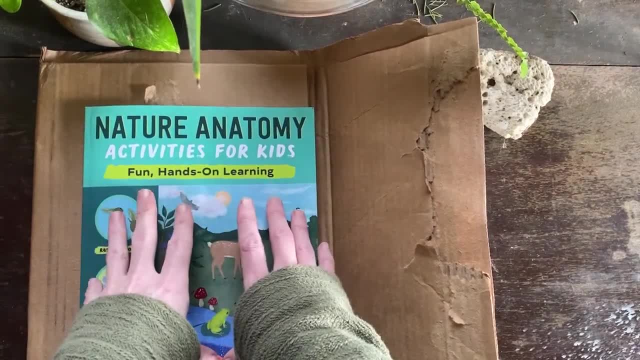 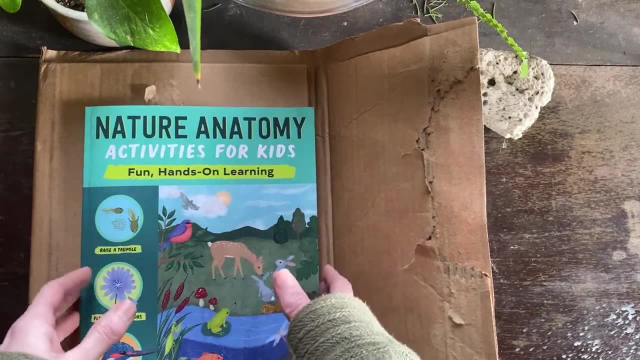 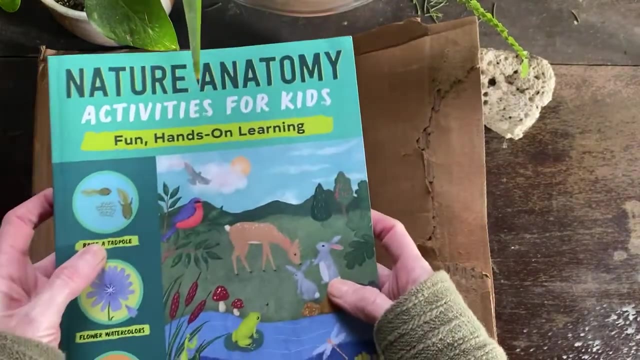 So your children will learn, will do an activity, And then they'll sit and they'll think about that activity that they did And they'll create a journal entry to help them reinforce that learning that they've just created from doing that activity. So it's on sale on January 19th. 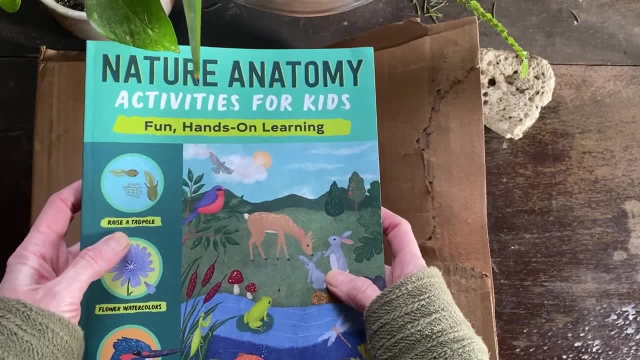 But you can pre-order it now. The link is in my profile.